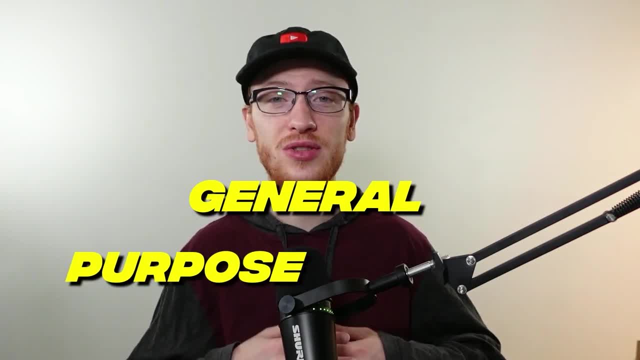 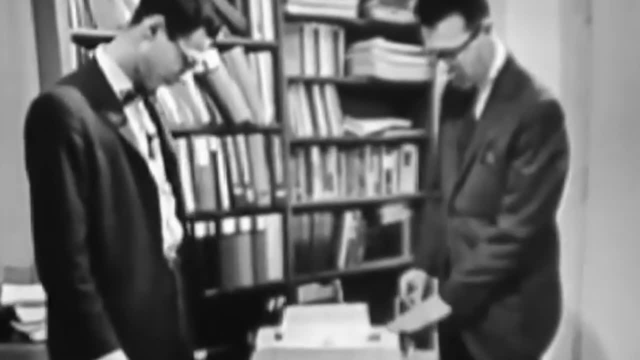 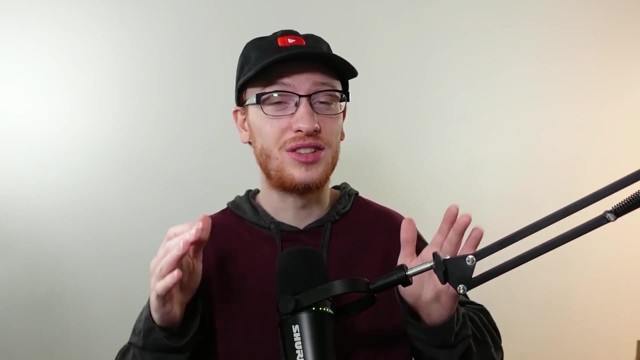 nailed it with basic. keeping along with this trend of general purpose languages, in 1972 everything changed. inside bell laboratories, dennis ritchie created the programming language that forever changed the world. you guessed it? it was b. okay, i'm just kidding, it was c, but it was called c because there was b and it was better than b. 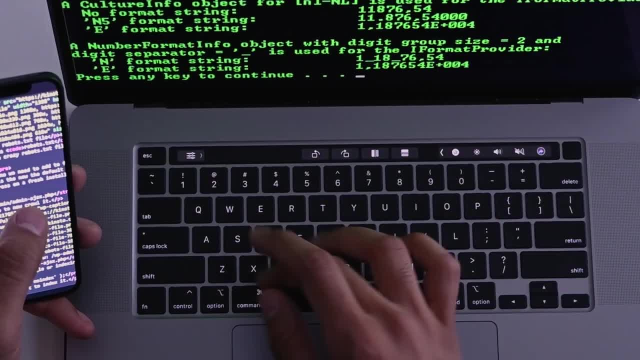 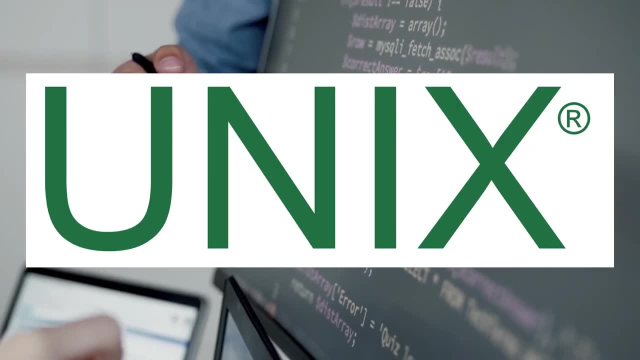 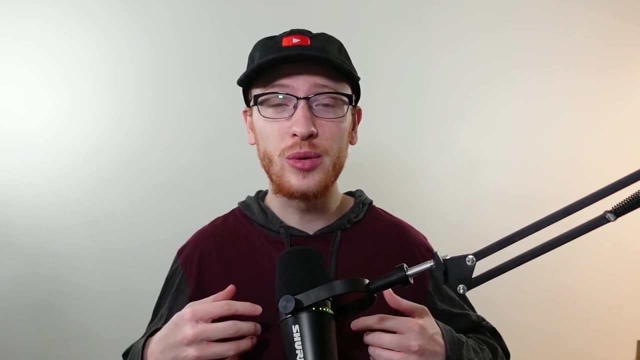 never mind. not only did c immediately become the go-to programming language for just about everybody, it was also used by the same person to create unix, probably the most important piece of software ever written. 50 years later, unix is still being adapted as both linux and mac os. that's right. 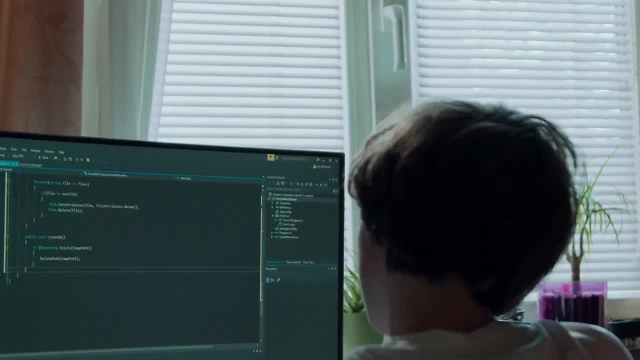 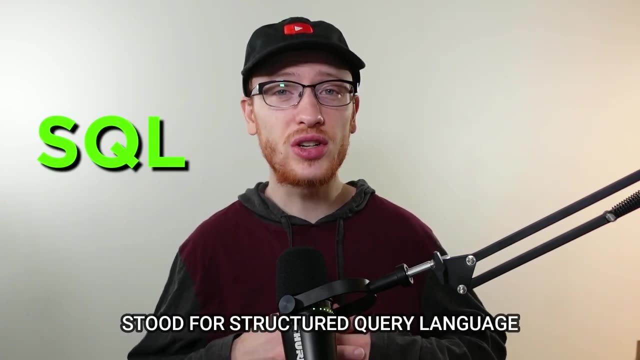 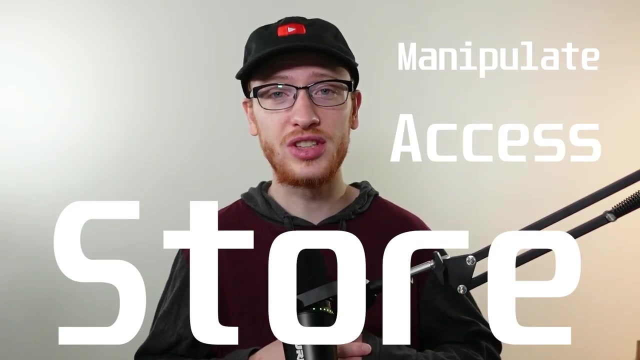 and the only other powerful computers are unix-based systems. if the rampage of the c programming language hasn't seen great enough, somehow, guess what else it made sql. sql stood for structured query language. it enabled pretty much everyone, as it was tremendously easy to use, to manipulate, access and store data in relational databases. it's just as popular today as it was 50. 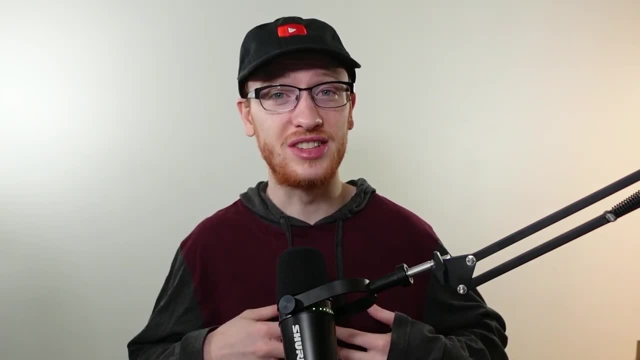 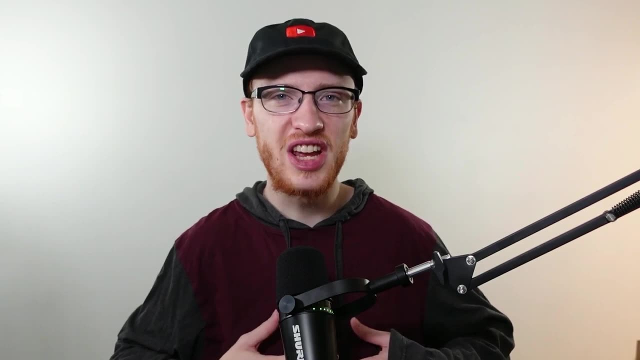 years ago. in fact, i'm actually a data scientist and the number one skill i'd recommend today is sql. oh, and another language that's coming up shortly. just one of the few that i'm using today is sql. wait for it. a decade goes by and c's onslaught was insane. you didn't need anything else, we had c for. coding and we had sql for databases. that's all you needed. however, as amazing as c was, it was also terrible. people today hate coding in it for a reason. one of those reasons is c strings. yeah, actually don't even get me started. there was many fundamental problems and there was phenomenal work. 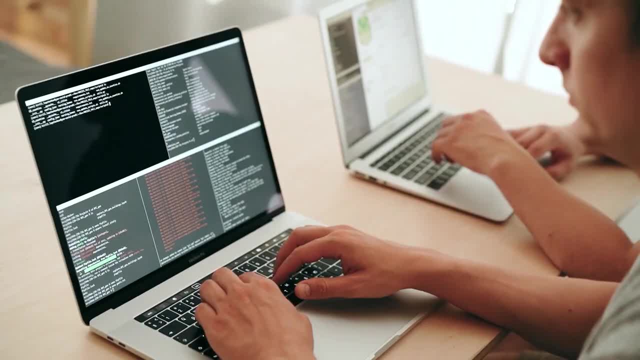 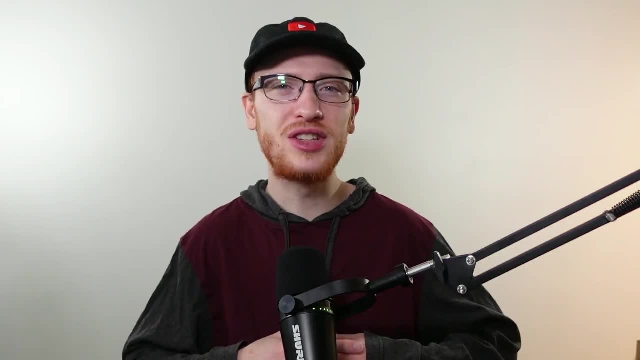 being done in the area of object-oriented programming, which made coding very, very fast. this is why, in 1983, bjarn strusip invented c++. c++ was basically c on steroids. there was a ton of new libraries, a bunch of fixes to its problems. 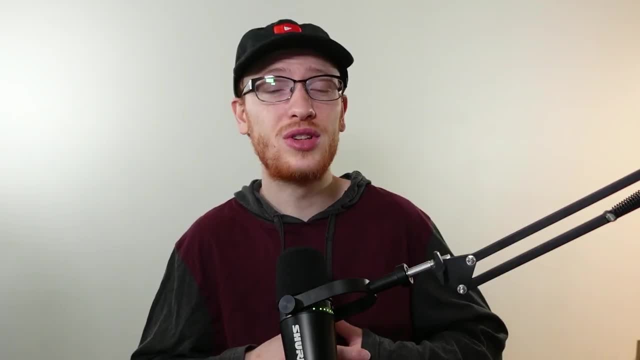 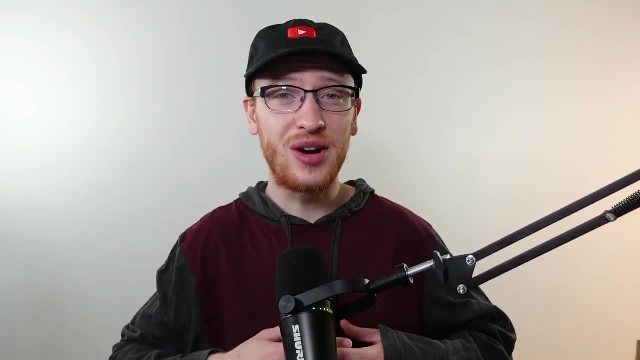 and it enabled this beautiful object-oriented design. while there's no massive problem with c and c plus plus, people just don't like coding in it. so in the 1990s there was an insane onslaught of new programming languages. the 90s gave us visual basic which allowed a drag and drop design of the 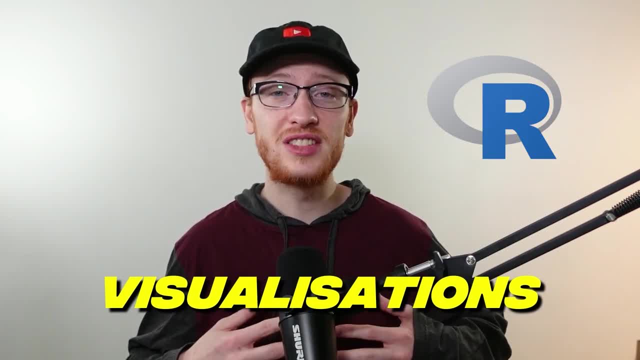 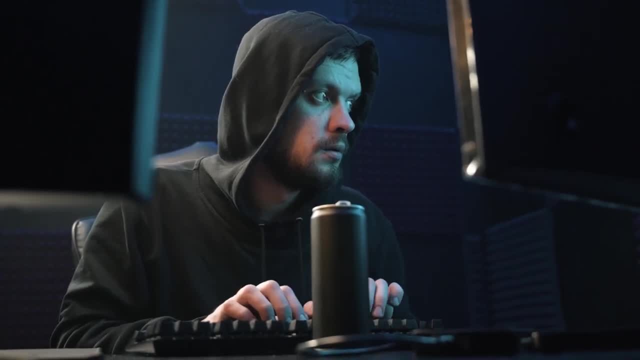 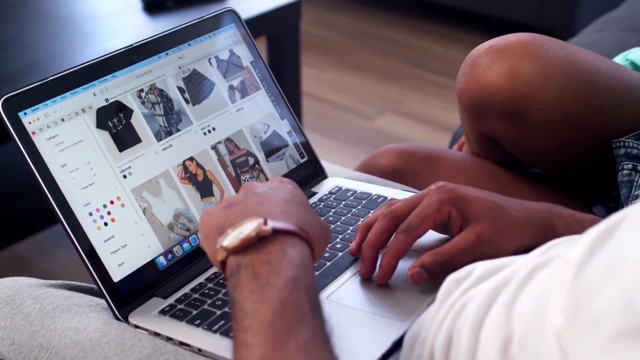 basic language. we got r, which made statistics and visualizations tremendously easy, like literally. we got java, which is basically just a better c plus plus. it's c plus plus without the pointers and it's on billions of devices. we got php, which soon dominated the back end of website creation.